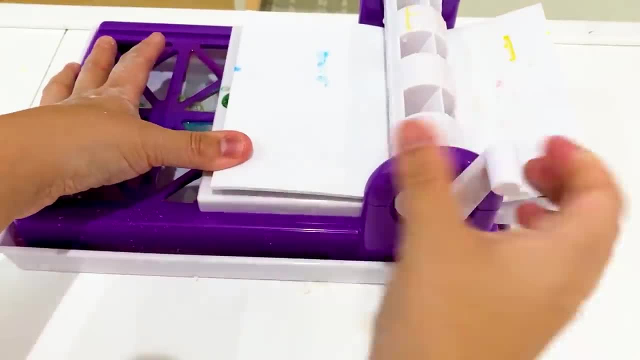 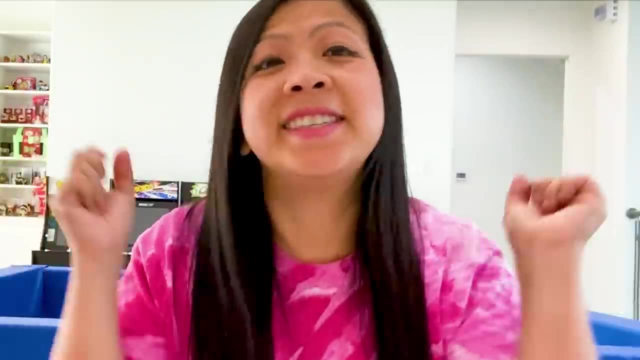 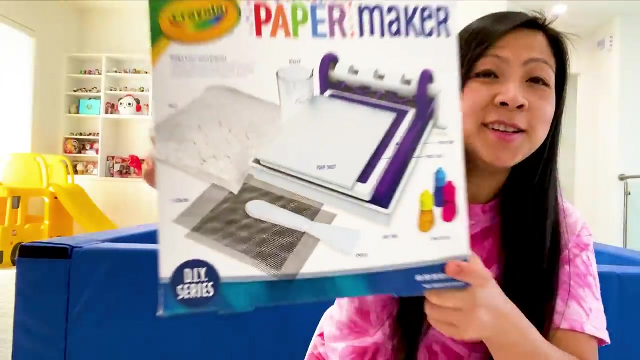 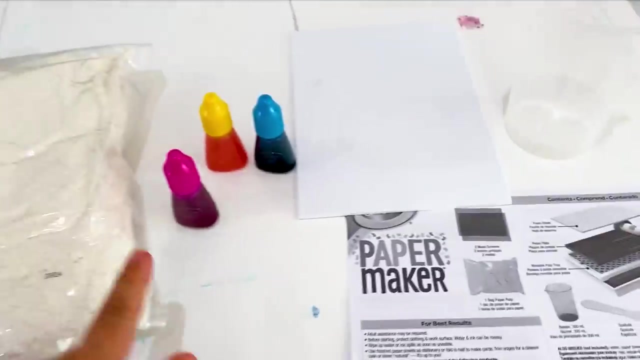 Come on, Flatten it, flatten it, Podgy family. Hey guys, today we're going to test out this really awesome paper maker from Crayola, So let's go and make some paper art. So it looks like it came with a paper roller, paper pulp, some food coloring, instruction paper foam and a 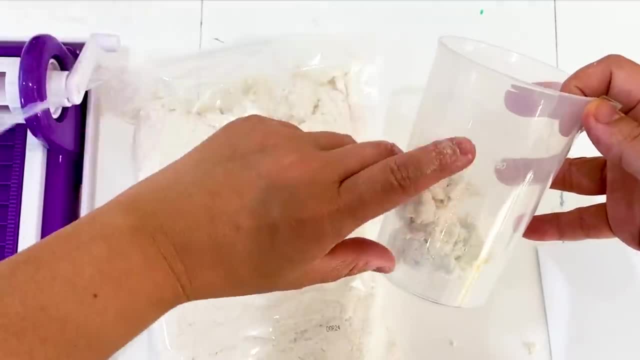 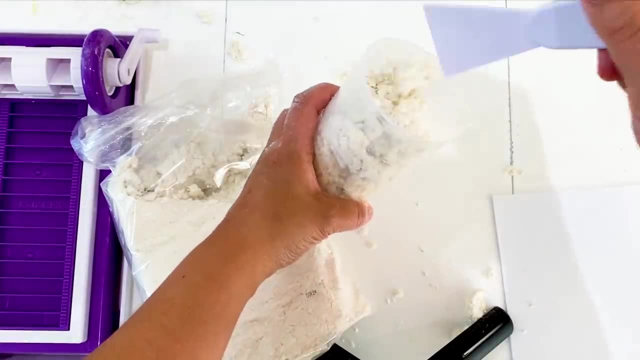 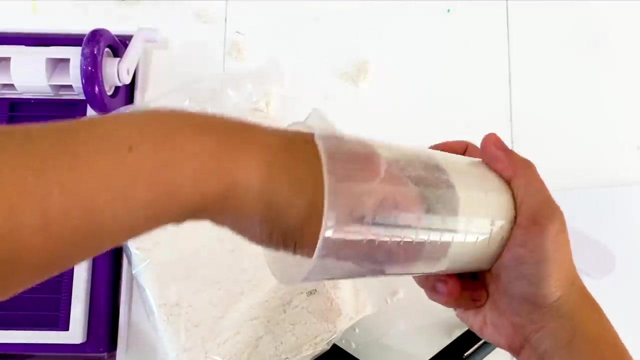 some paper pulp to the beaker, to 250, right there, Oh whoa. Look at this. It looks like a shredded paper, almost Okay. and then we're going to use the spatula to just make sure it's squeezed down. Squeeze, squeeze, squeeze, Flat, flat, flat, Okay. so I'm actually supposed to. 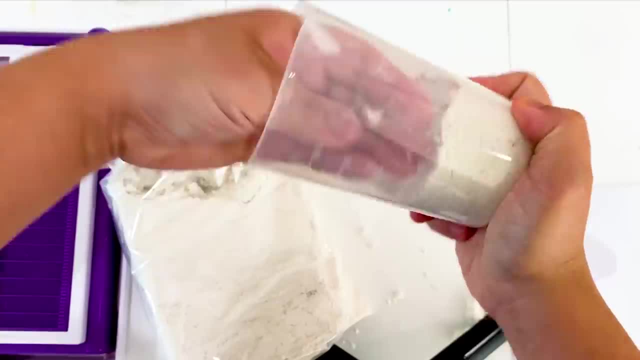 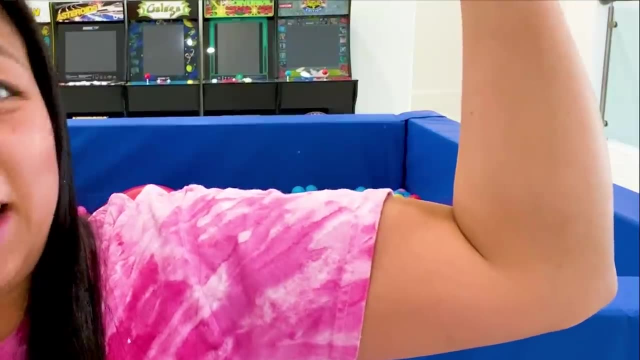 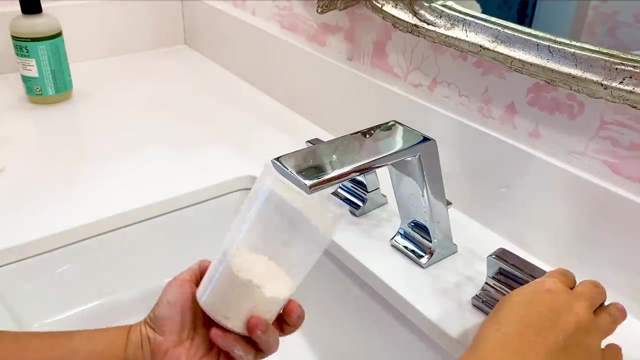 just squeeze it and press it all the way down until it reaches around 75.. This looks a lot harder than it is. I don't have the strength. Look at this. That's not muscle. Okay, I think this is good enough. Oh, that's on my face, Okay. next, it's said to add: 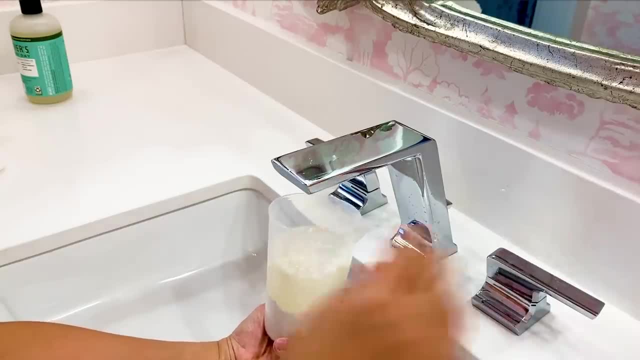 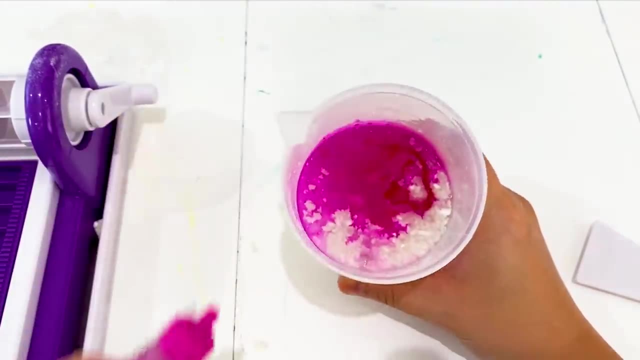 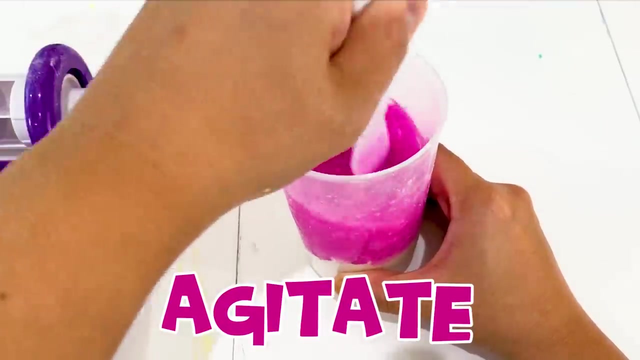 water until it reaches 250.. There Next it's said: add some color. I'm actually going to use some pink Whoa, looking bright already. Then it says to stir. Another word for stir is agitate, So I'm. 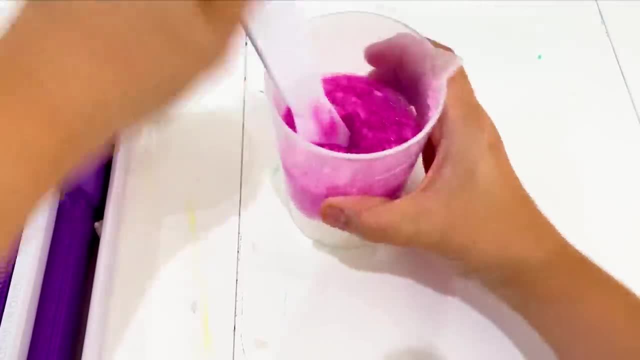 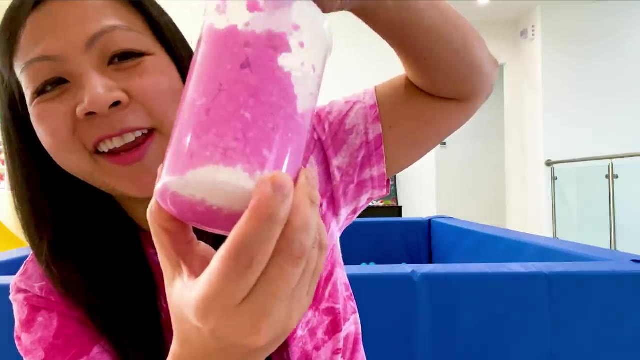 going to agitate. We're going to agitate all this pulpy paper. Okay, what do you guys think? I think it's pretty much up. Oh, I missed a spot. Never mind, I thought I got it, but I didn't got it. Okay, we're. 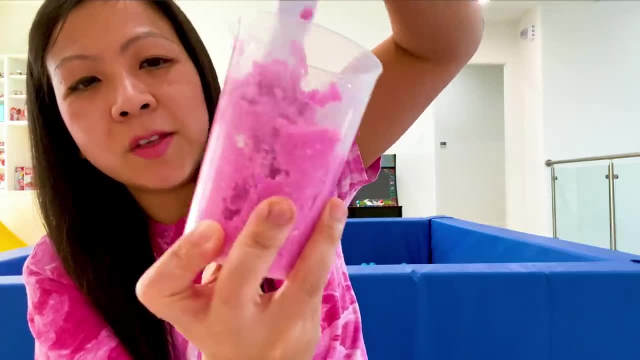 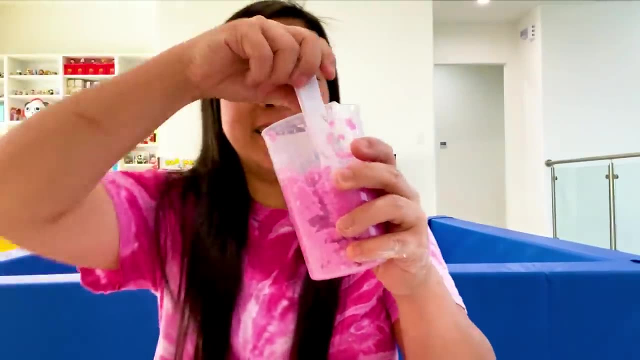 going to keep stirring and agitating until I get all of it to become pink. I think we're almost there, you guys. Oh, look, the same color as my shirt. If you guys don't know, my favorite color is pink. What about you guys? Okay, I think it looks pretty good. 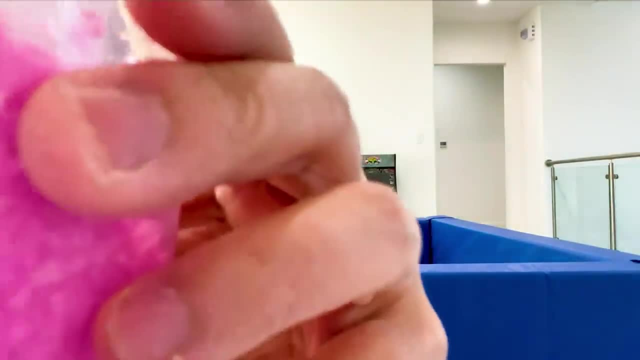 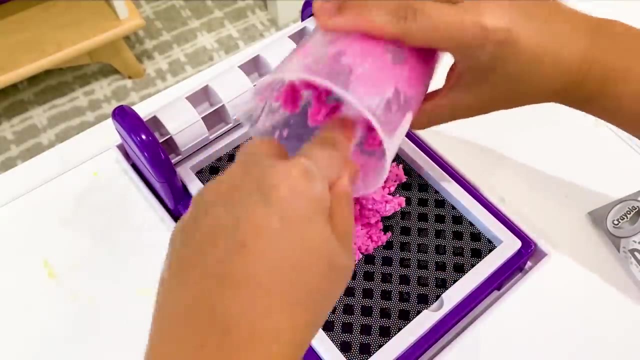 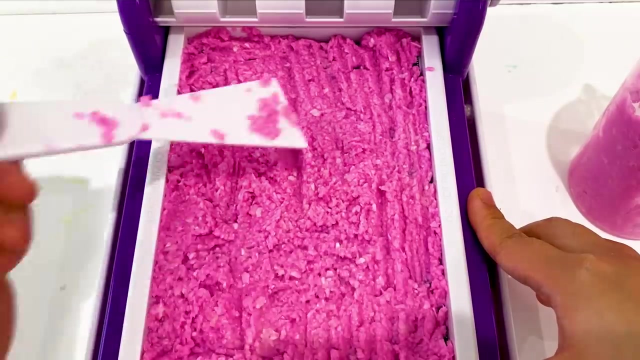 All. right on to the next step. Woohoo, Oh, can't, It's on this side. On to the next step. Woohoo, Okay. next step is to pour the pulp here and just spread them. I really like this. What do you guys think? Okay, when it's done, it says: put the mesh. 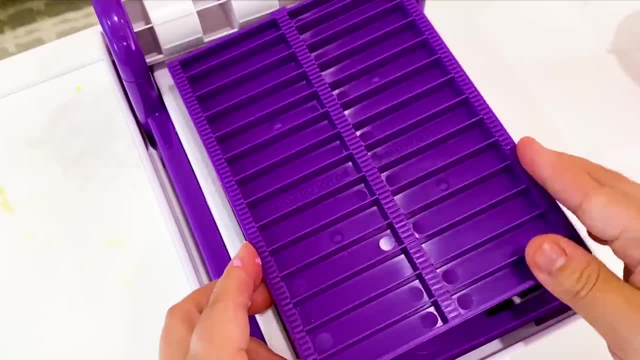 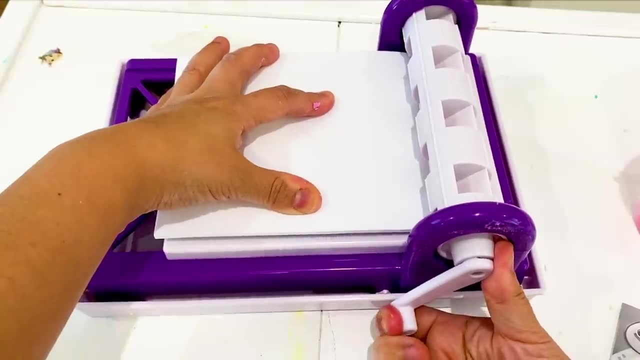 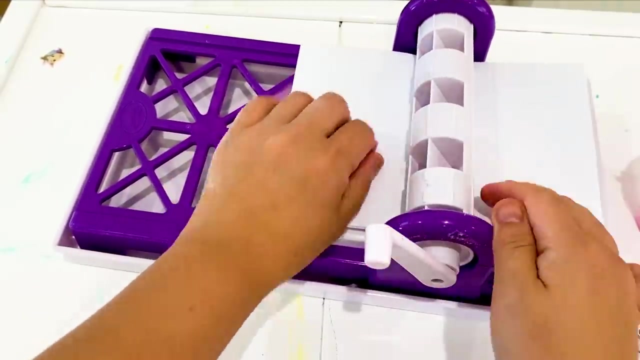 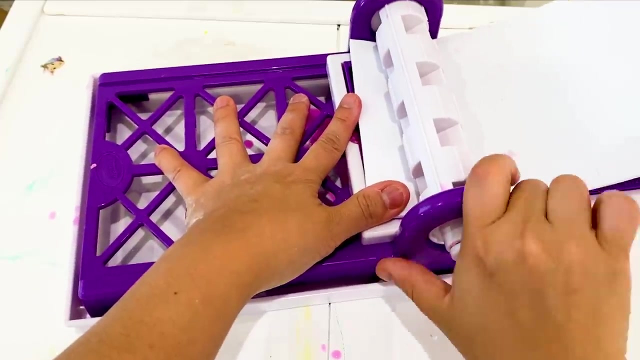 on top, then this on top, then the foam on top of that. Okay, next thing they say to do is to roll the paper. So we're going to roll. This is harder than I thought. Okay, it says to roll back into its original position. 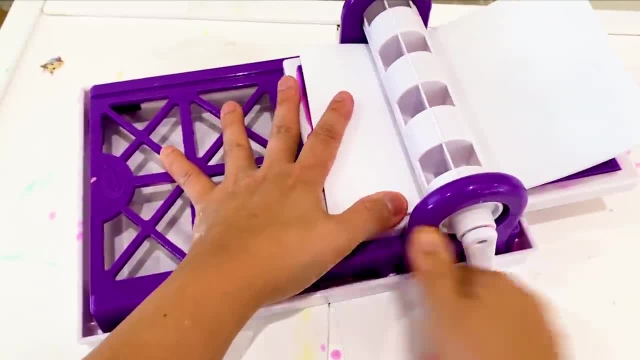 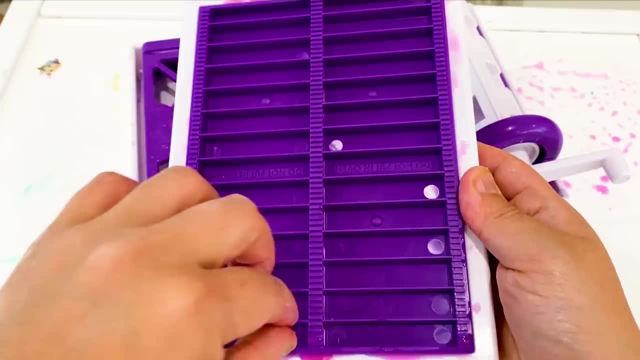 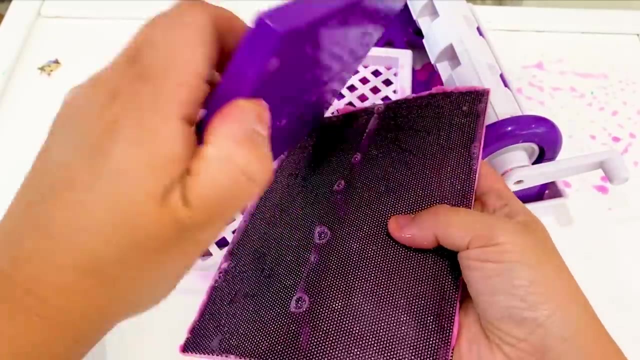 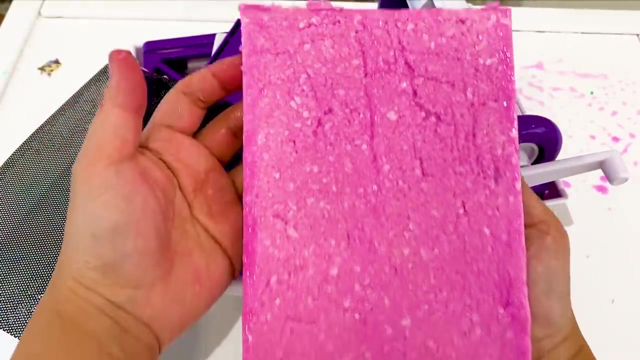 The other way. Oh wow, I am just way too weak for this. Okay done, And it says to remove it. I'm Ready to open this. Oh wow, A little bit of that. Oh wow, Woohoo, Whoa, look at that, That's. 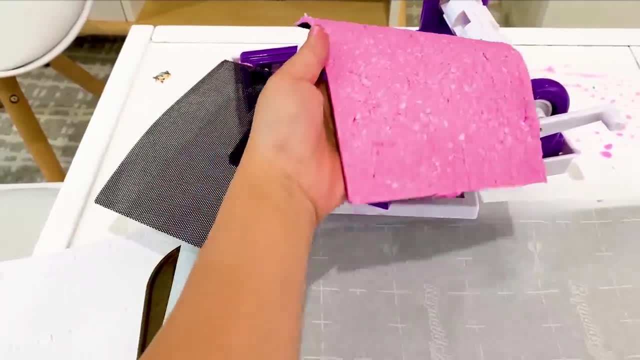 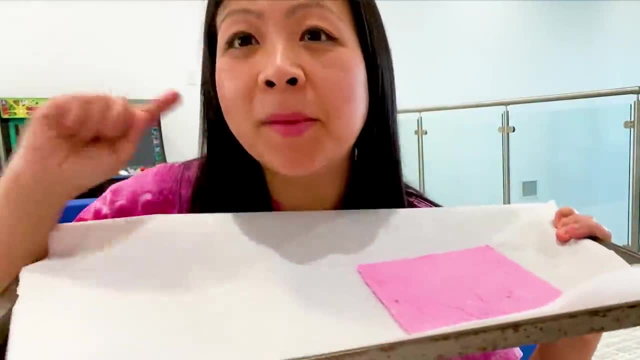 really cool. Okay, so my paper I'm going to put here. Okay, this is the coolest thing. That is so cool. I'm going to make another one, but this time multiple colors. okay, Okay, version two- again in his suit. I'm reading a arribie read through my book about my favorite books all over the country And I will stop. Valejo, It's an awesome book. That's great. Good, Yay, It's incredible. Thank you all so much for watching us. I'm such a romantic, Michelle. I love you all. Cheers, Bye-bye. 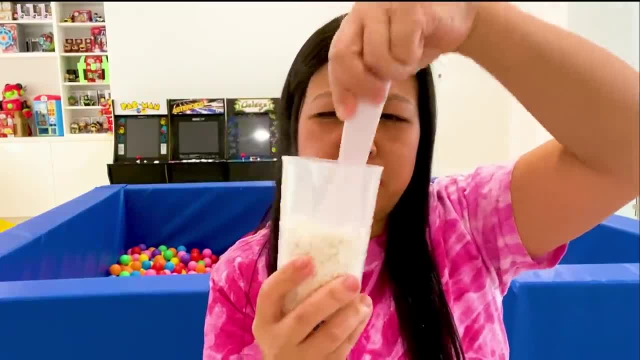 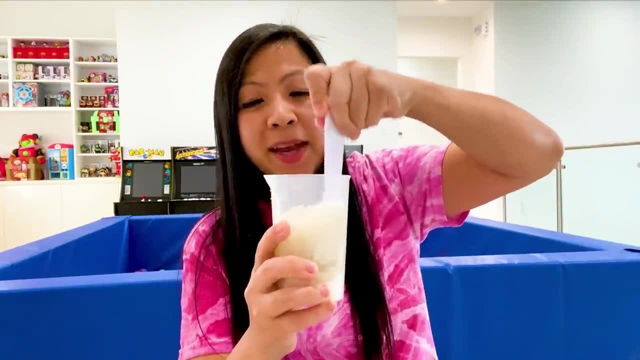 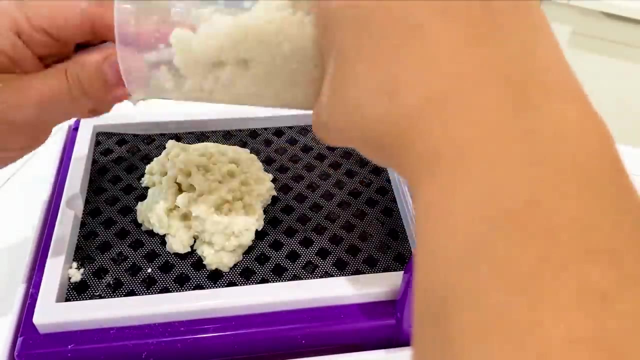 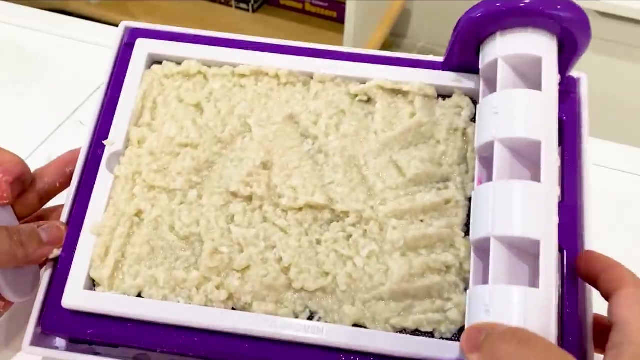 again, add paper, press, press, press, press, press. oh, i'm just gonna use my hand. add water, stir, stir, stir, mix, mix, mix. this time i'm gonna keep it white, okay, and then i'll add color. while it's in the paper roller. let's put it on, spread, go, okay, done. next, i'm just gonna add some drops of colors. 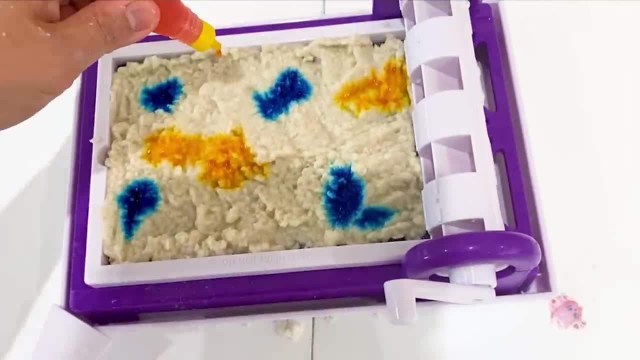 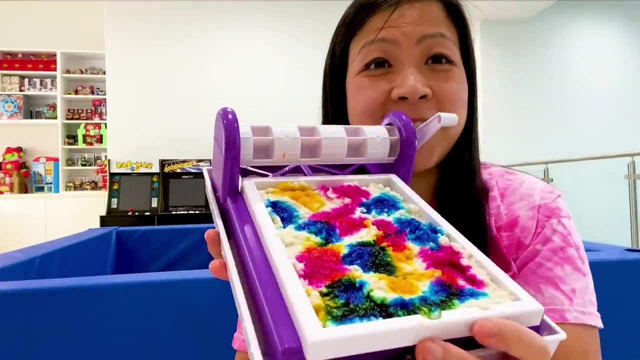 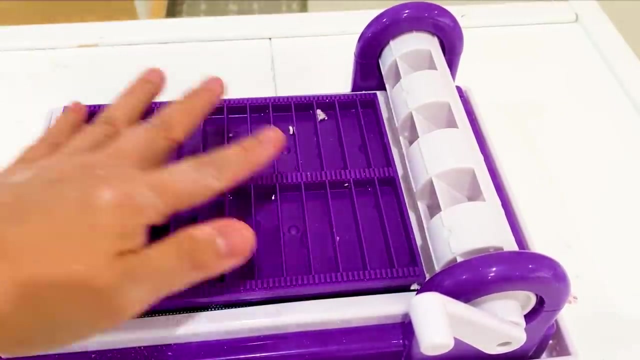 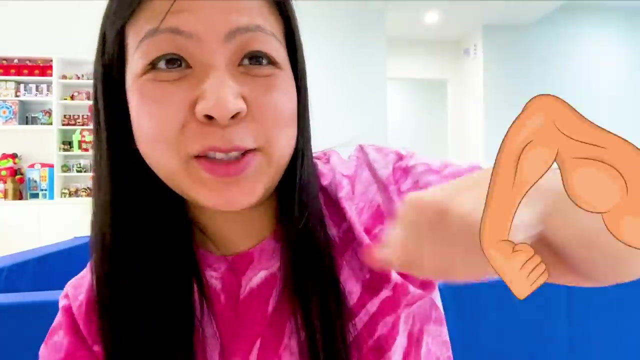 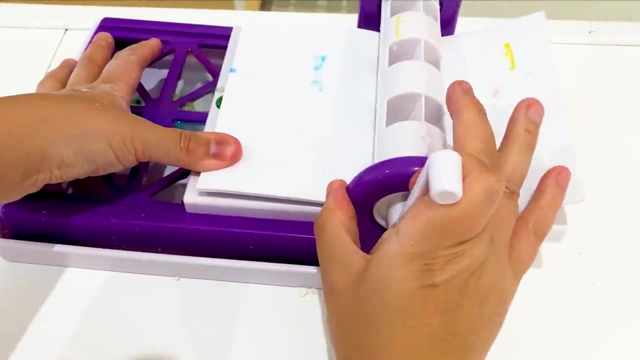 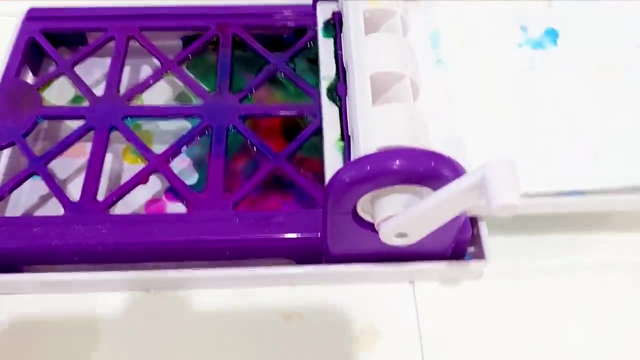 look, oh, that's really cool. what do you guys think? done. okay, that is so beautiful. okay, next the mesh paper, this other thing- and the foam. next, using all my strength, let's roll it. who am i kidding? what strength, come on, flatten it. flatten it. there we go. okay, i'm doing it. yay, oh, look at the color inside there. okay, let's. 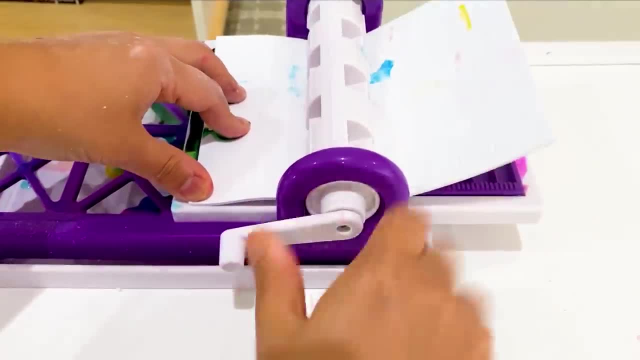 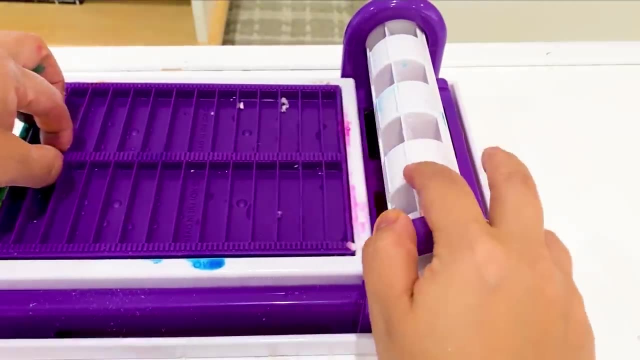 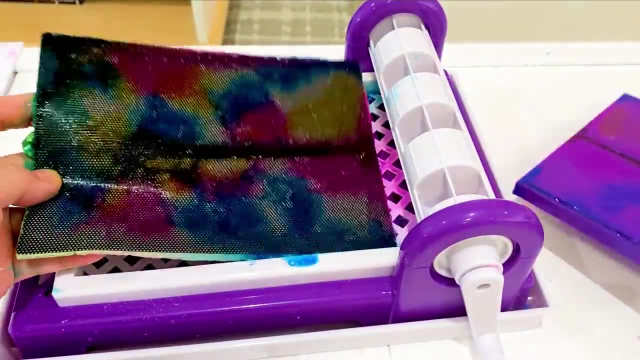 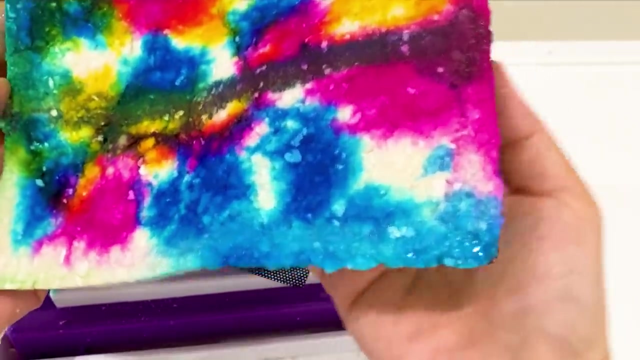 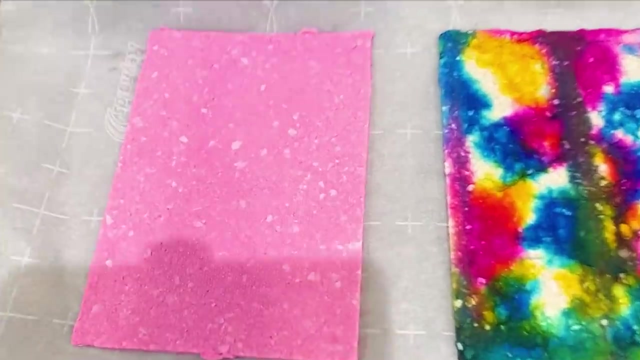 roll it back. come on, okay, all right, let's check out our awesome creation. there we go. okay, got it out. okay, did we do it? oh, whoa, moment of truth. oh, that's pretty. look at that. okay, this is a fancy paper. okay, guys. so there it is our first pink paper, our